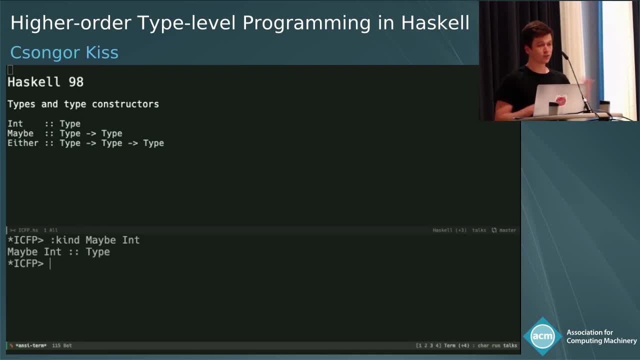 indeed it gives us type. Now these type constructors can be partially applied as well. So when I ask GHCI what the type of, so what the kind of either of int is, it'll partially apply either to int and we get back something that has kind type to type. So why is partial? 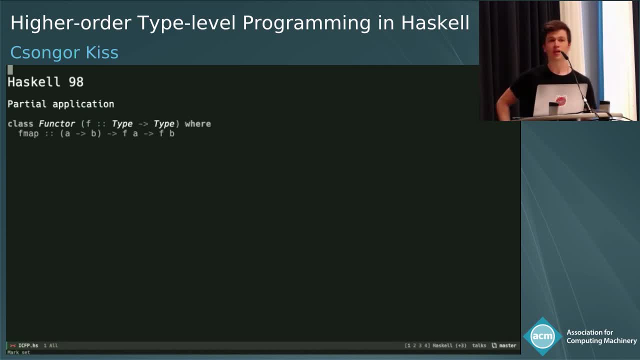 application of type constructors useful Well as an example. Haskell has a lot of this type class called functor, which allows us to abstract over types that have a type parameter, such as maybe an either, and in this case, the functor type class gives us a way to. 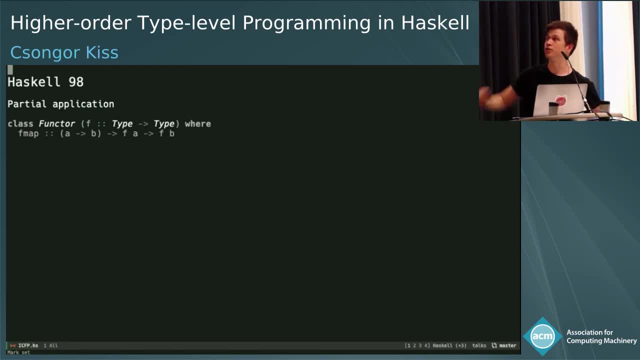 swap out that type parameter with something else. by giving a function A to B, We can go from F of A to F of B. So here are two instances for the type constructors we've seen, maybe, and either E, and notice that I had to partially apply either here because 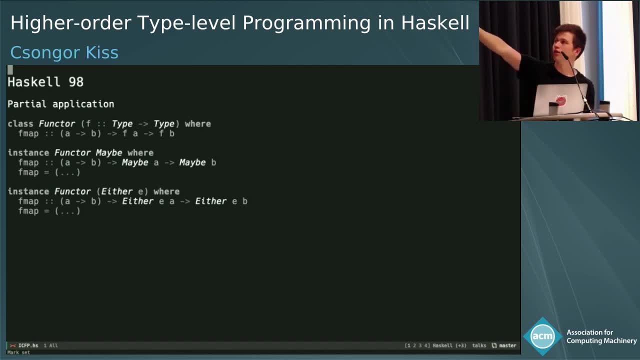 normally it takes two arguments and the kind of the argument of functor is type to type. So that's good, Haskell 98.. How does type inference work? We all know that Haskell has very good type inference, so we expect to be able to just use these functor. 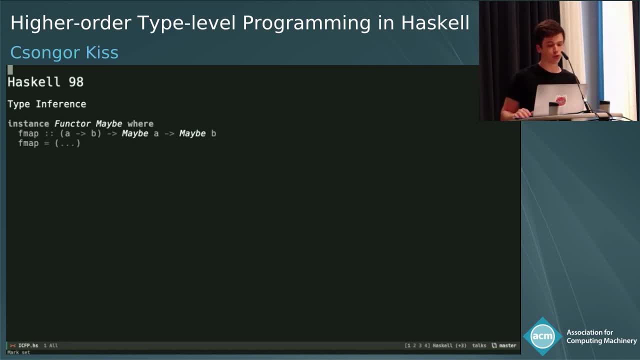 instances without having to provide any type signatures when we do so. So here's an example of using fmap on a value of type maybe bool. We call fmap show on a value of type bool and if we ask what the type of that is, it should be maybe string. So GHC cleverly figured out. 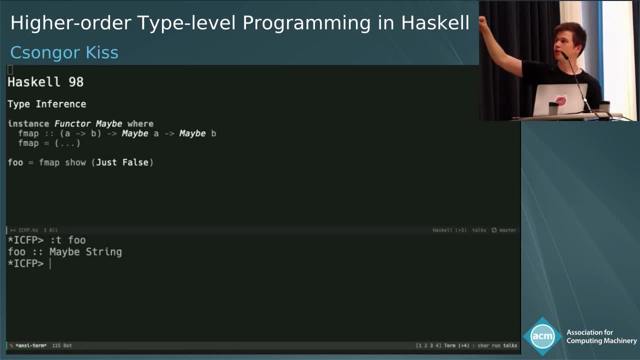 that, going from maybe bool, you can with a function, bool to string, we can get to maybe string. So how I did, how we did this? well, a very important thing that GHC does during type inference is application decomposition. So we start out with the type fmap: A to B to F, of A to 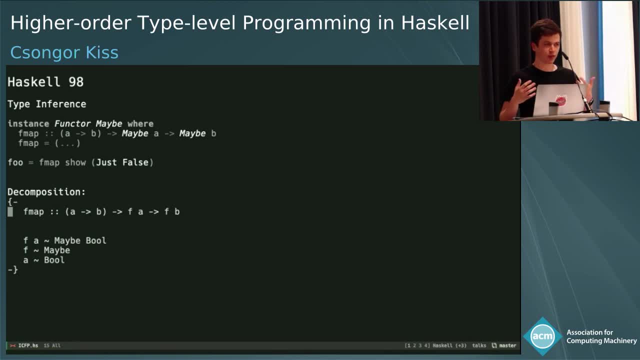 F of B, And GHC sees that we passed in a maybe bool as the F of A argument, so it sees that that's an F of A equals maybe bool and it. behind the scenes it decomposes this application and discovers that F must be then equal to maybe and A must be equal to bool. So the 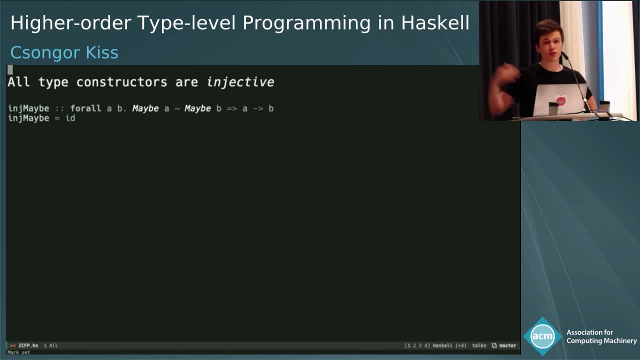 GHC does this during type inference. As a result of this decomposition, it turns out that all type constructors in GHC are injective. So what that means is we have this function here with a context that says for all A and B. if we know that maybe A equals maybe B, then we can. 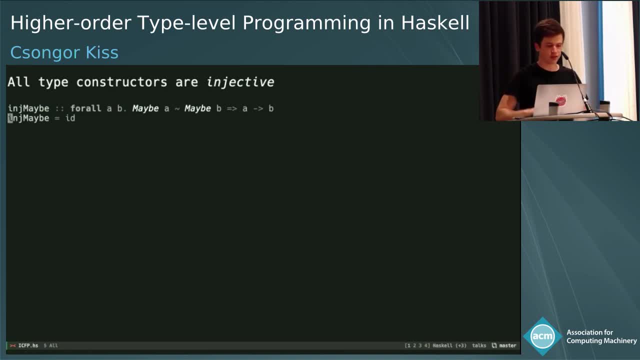 write a function A to B and implement it as the identity function, which is only possible if we somehow in the process manage to learn that A must be equal to B, because the identity function doesn't change the type. So maybe it's injective And actually every type constructor in Haskell. 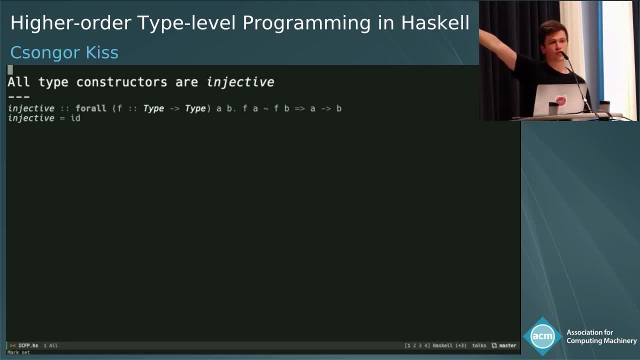 is injective. So we can even abstract over A to B and we can write a function A to B and we can work a super- Hugging역 of this phrase, for some reason Over- over a, maybe from the previous. 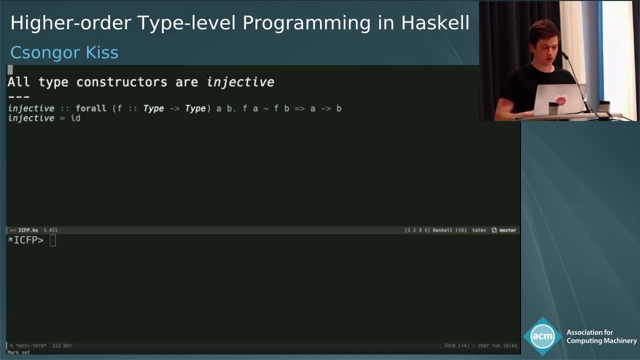 example, and should say that any F of this kind type to type is injective and this still compiles as we expected. And indeed if we say we'll look at the type of injective instantiated with with maybe for F, so we can use visible type applications to provide maybe. 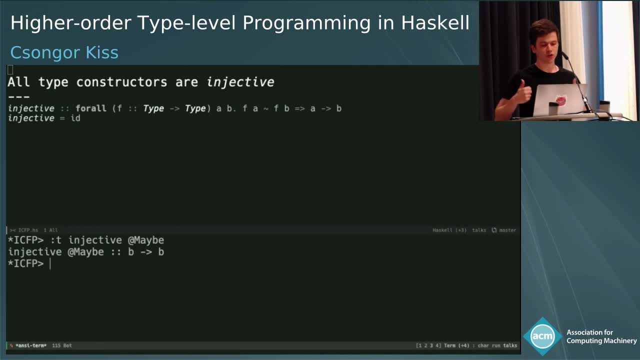 as the, as the argument F. So just GHC will indeed tell us that. oh yes, I learned that we deal with this dulu than we later talk about in the скорare. But perhaps you know, since our design is very different from what we've seen before, our design is different from what we've. 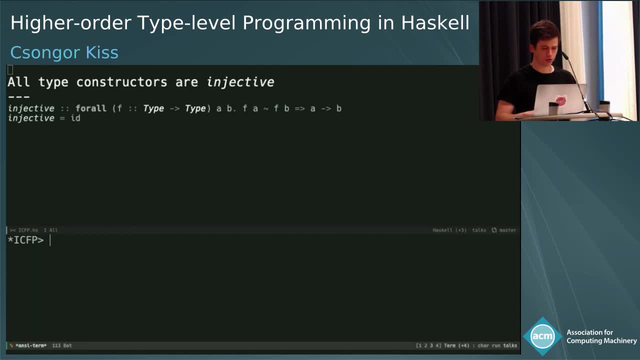 data and in terms of what is that designed? so to develop these? you know a lot of data management, that the A and B must be the same. So all type constructors are injective And all type constructors are also generative, which is the other property that is implied. 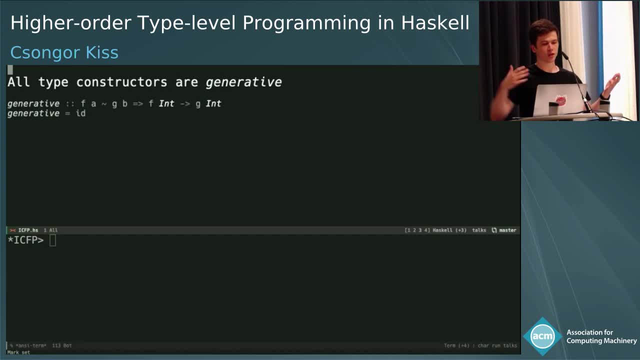 by application decomposition. So when we saw that F of A equals maybe Boo, we learned that A equals Boo, which is the injectivity property. Being able to learn that F equals maybe is the generativity property. So in this case, when we know that F of A equals G of B, 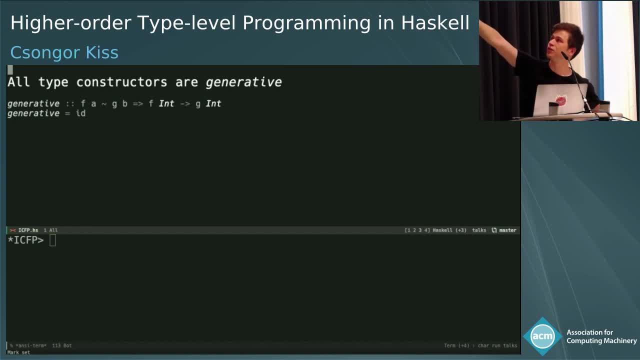 we can again write the identity function and type it at F of int to G of int, because GHC learned that F must be equal to G. So this is pretty standard Haskell 98 type inference. So again just to recap some of these definitions. 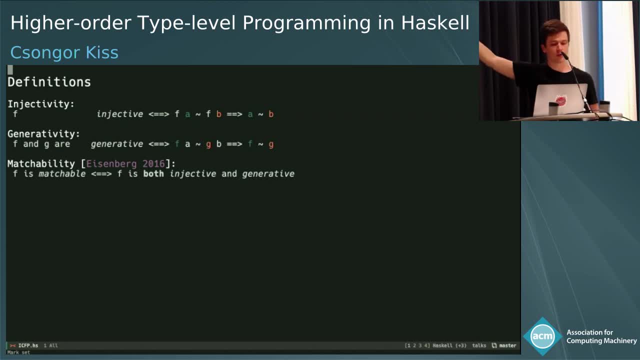 injectivity means that F of A equals F of B implies A equals B, And generativity, in this case, means F of A equals G, of B implies F equals G, And so when something is both injective and generative, then we can call it matchable, which? 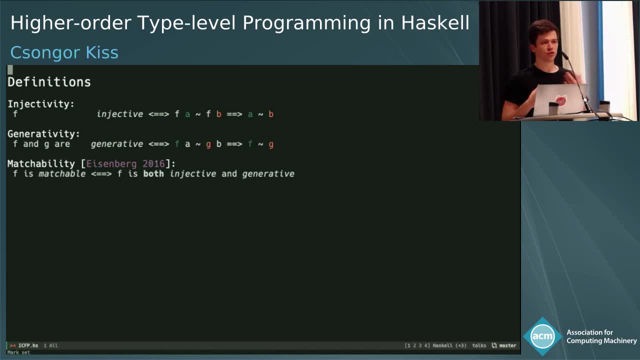 is a term. It's a term that characterizes the way type constructors are handled by the type checker. OK, So let's get back to the future. So far we've been talking about Haskell 98.. Now for the rest of the talk. I'm 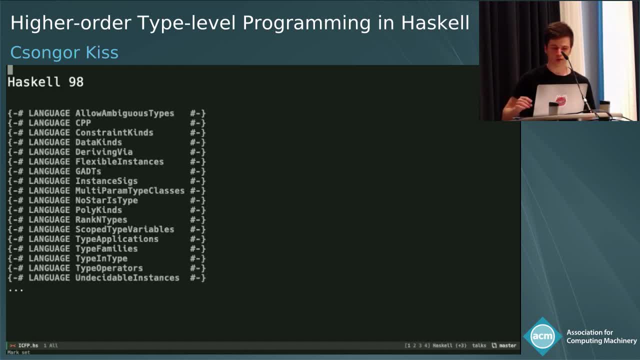 going to talk about Haskell 98, but with a different meaning of the word, that is, Haskell with 98 GHC extensions turned on, And in particular, I'm going to focus somewhat on type families, which are just down there at the bottom. So type families are a way of, as we've seen before, 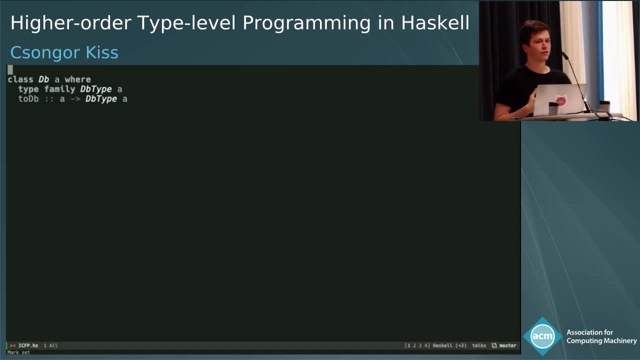 type families are a way of expressing computation at the type level in a functional way. So what I mean by that is, if you look at this example, we have a type class here called DB, which is intended to represent types that have a database encoding. 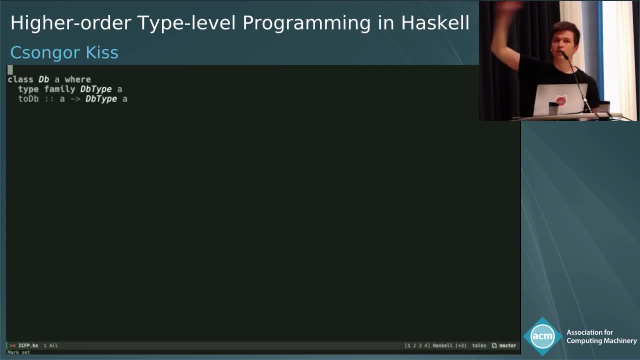 somehow. So we can see that in type class DB there isn't, you know, a, an associated type family called DB type which sends a type A into its DB type. So whenever we instantiate in this type class that we need to provide for every type their DB type, 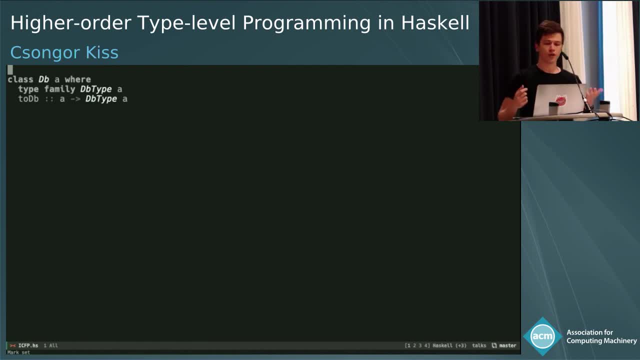 representation. there's a function to DB which then hopefully does the serialization to the Haskell type, to the database type. So you can see that very similar to maybe, and either DB type also has a kind type, arrow type. So just keep that in mind. 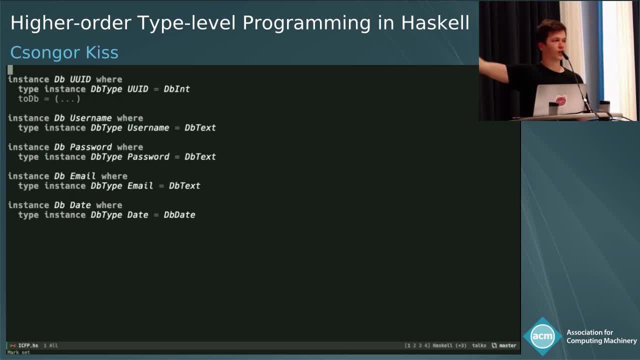 So a few examples here, taken out of an enterprise Haskell production code base. You can see it's enterprise, because username and password are both mapped to plain text in the database. So this is what type family definitions look like, And indeed we can again jump back into GHCI. 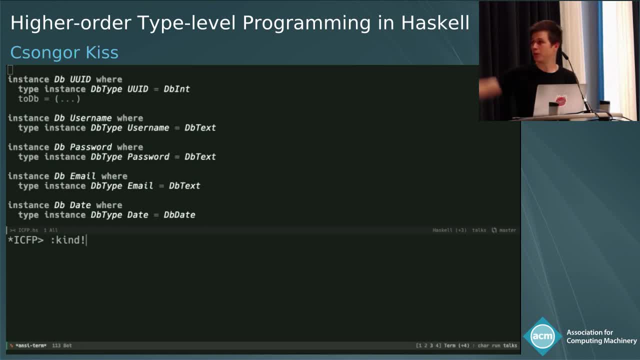 and evaluate these type families. This time we put the bang at the end of kind which tells GHCI to really reduce the definitions, And indeed we can see that DB type password reduces to DB text. So we've got a nice type level computation machinery. 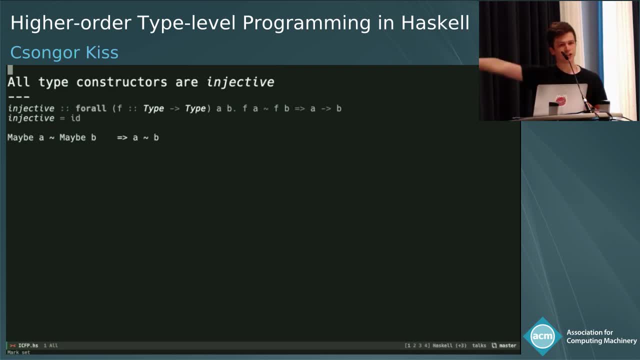 in our hands. But let's just go back to the injectivity property for a second. that we've seen. So every type constructor in Haskell is injected, which means that we can instantiate the injected functions F argument with any type constructor and it'll just work out. 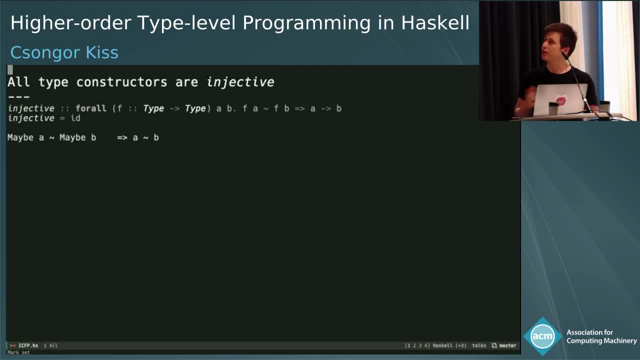 It'll tell it'll, it'll know that A must be equal to B because the, because of the context. So in the case of, maybe this worked out. But of course, if we think about the DB type type family, this property really doesn't hold true for it. 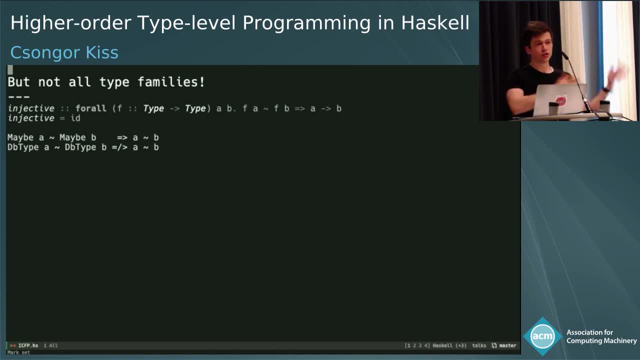 because DB type of username is equal to DB type of password. But we really don't want to be able to learn from that that username is then equal to password. So DB type is not injective, nor it is generative, it turns out. 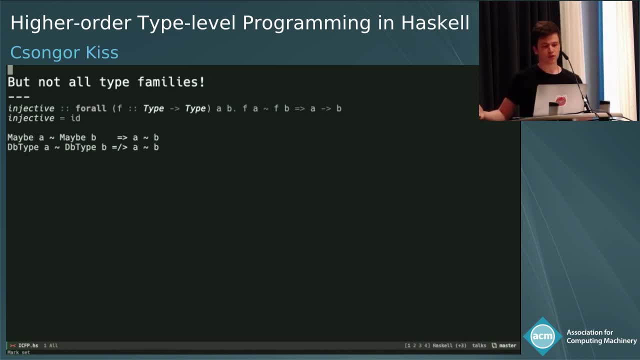 So today in GHC, what happens when we try to try to instantiate injective, just like we did with maybe what if we try to instantiate injective with DB type? So really wish this didn't work. And indeed GHC tells us that the associated type family DB. 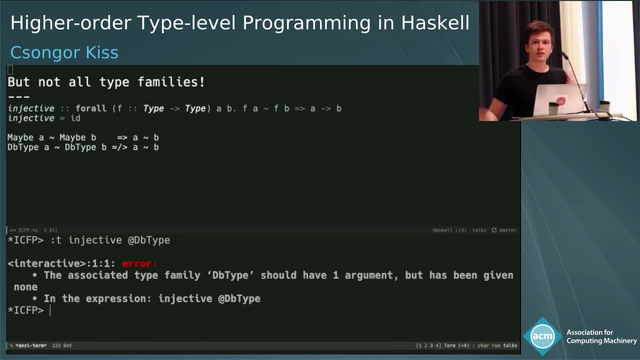 type should have one argument, but has been given none. So the defense mechanism in GHC is that it simply doesn't allow partial application of type families, because if it did, then well then we could do nasty things in this way. So OK, type families must then be saturated. 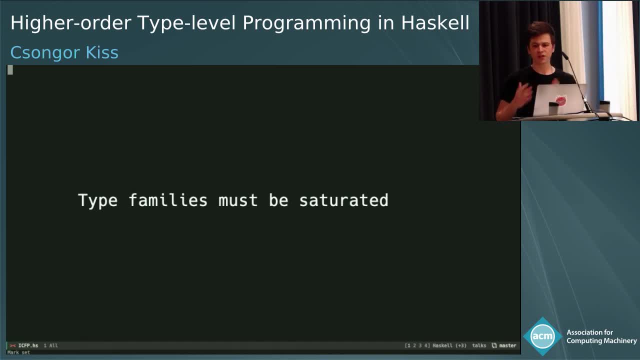 This is the rule today in GHC And in the next couple of minutes I'm going to show an example where this restriction is really quite restrictive. I'm going to motivate why we really want to do unsaturated application of type families. but let's not get ahead of ourselves. 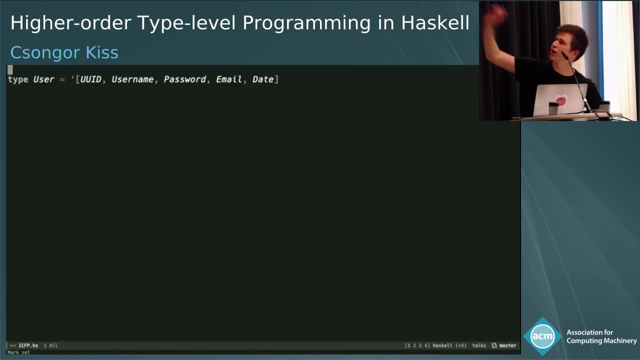 So again, Haskell 98,. this is a type level list. So whenever you see a tick, it means that this constructor is now promoted to the type level. So lists exist at the value level, but tick lists exist at the type level. 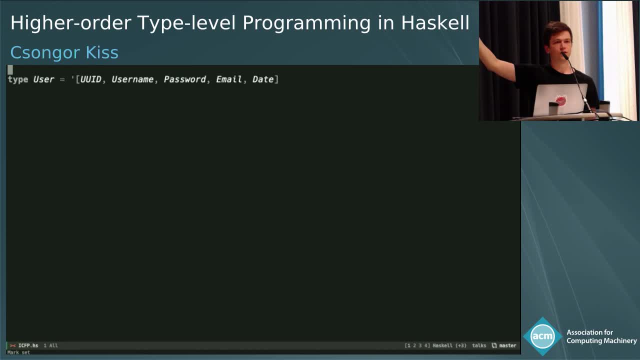 So the user type is a type level list of these fields that we've seen earlier. So every user has an ID, a username, a password, an email and some registration date or birth date. Now, in order to have a value that somehow inhabits, 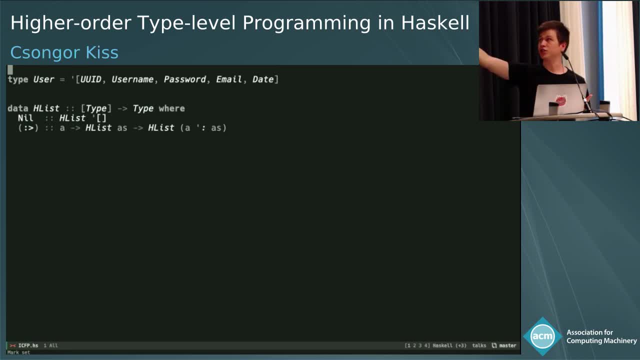 this shape of data we can define a heterogeneous list, which is a generalized algebraic data type indexed by a type level list. So what that means is we can have a list whose elements are all of different types, and these types are given by the list. 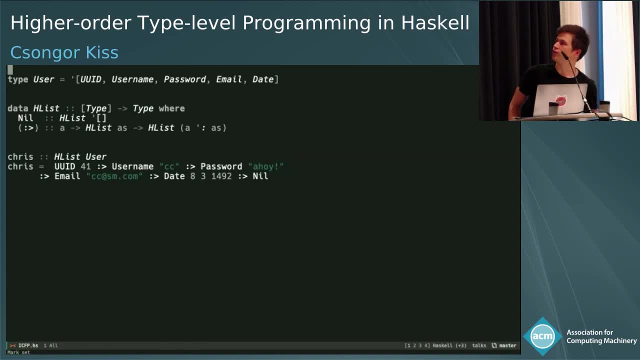 So in this case, we can see that our user Chris is a user which is implemented as a list. Every field has a different type. So what? What if we wanted to take a user list and turn it somehow into a database list? So again, this is the definition of the user list. 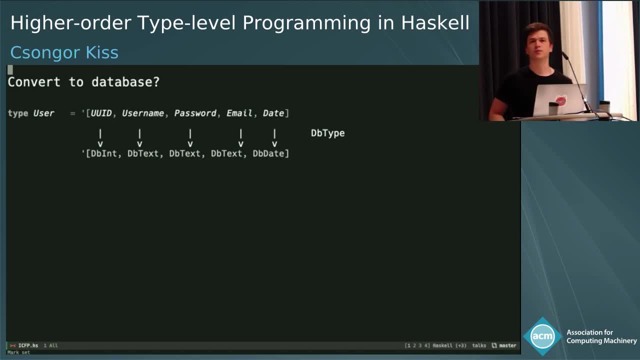 And somehow we want to end up with. so, given this list, we want to end up with a list where every field has been turned into the data type equivalent of the original type. So a function that does this might look like dbzer of type. 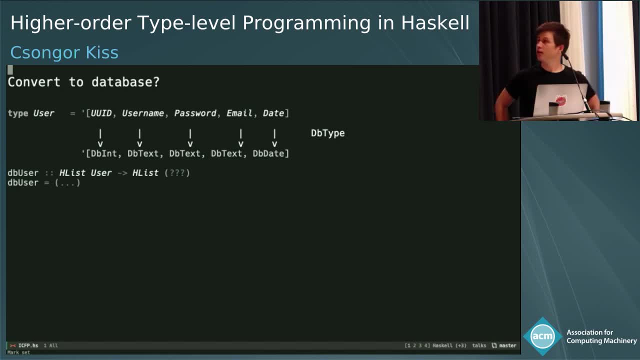 list. So we can change this from agelist user to agelist. and then what? So at this point we can say, OK, we're just going to hard code the result of this mapping, But the problem with that is that every time then 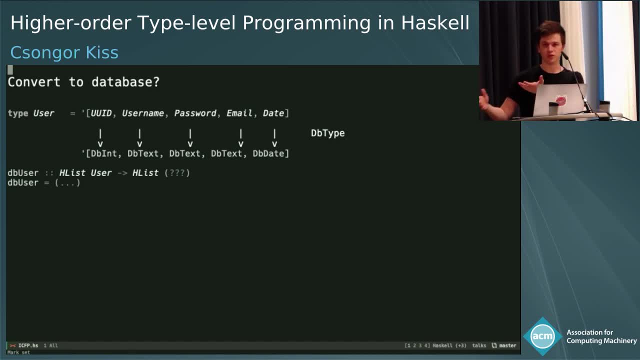 we extend the definition of user, we also have to update the type of the dbuser type, So it's kind of unfortunate. What we really want to do is somehow lift this subtraction out and do this in a higher level way So we can go and define a type family called map, which is the exact same function as map at the value level, but everything has been turned uppercase, which means it's now at the type level. 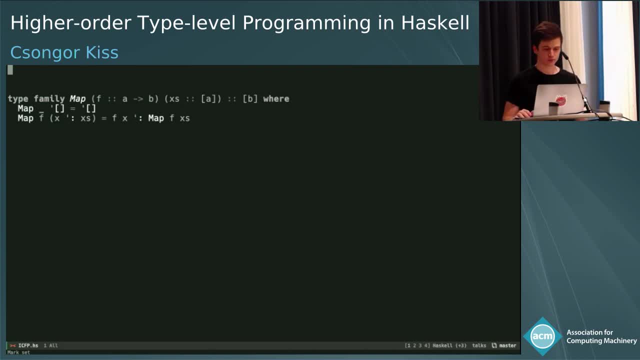 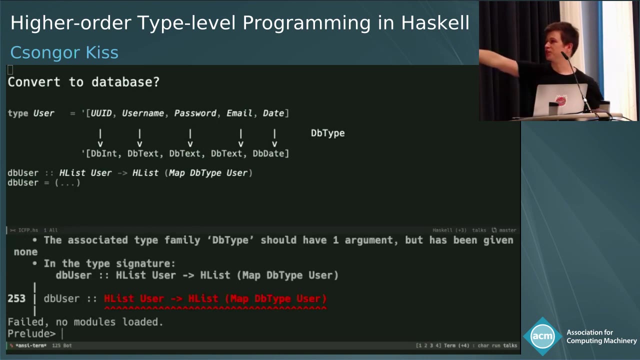 So it goes through a list and applies a function and translates the values. Okay, so we go and say agelist map, db type over input, over user, And we try to reload And again GHC tells us that the db type is partially applied. 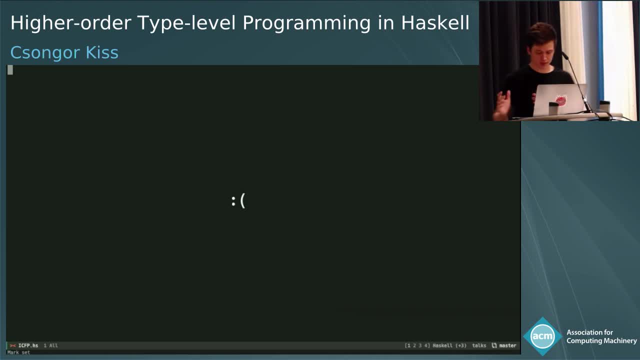 So that's no good Sad. Okay, so the first idea, which is due to Richard Eisenberg, is that if we want to keep type inference behave as it already does today, but also do type level partial applications, then we're going to have to do a lot of things. 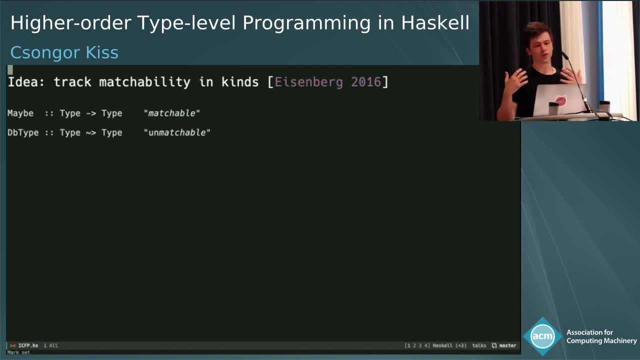 So we're going to have to do a lot of things And we somehow need to distinguish the kind of type constructors and the kind of db type in a first-class way in the type system. So what we're going to do is we keep the kinds of type constructors as they were. 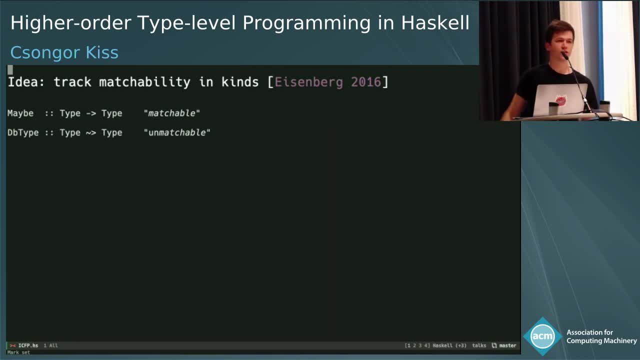 but we're going to assign these squiggly arrows as the kind of type families, And so the normal arrow is pronounced matchable arrow and the squiggly arrow is pronounced unmatchable arrow for reasons that are not, And so the normal arrow is pronounced matchable arrow for reasons that are not. 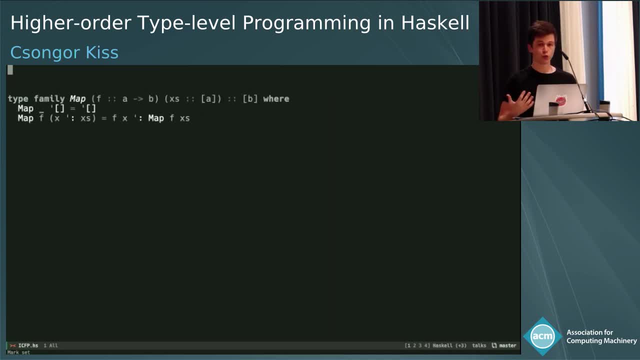 And so the normal arrow is pronounced matchable arrow, for reasons that are not, Hopefully, clear by now. So how do we then fix the map function or the type family to accept type families as arguments? Well, we just replace the arrow with a squiggly one, with an unmatchable one. 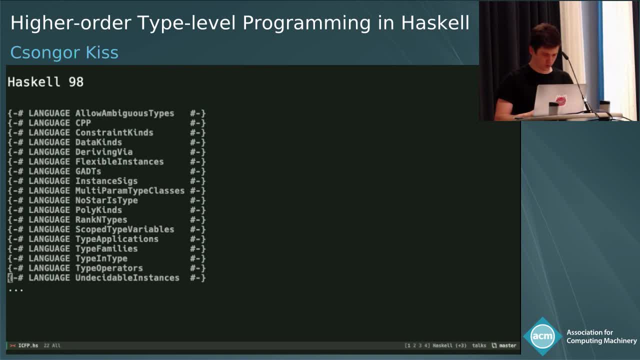 And, of course, because this is a new feature in GHC, we need to add another extension called unsaturated type families, And I know what you're thinking now. Okay, well, this takes This takes us into Haskell 99 world, and it was already quite difficult to deal with Haskell 98, so it's really no good. 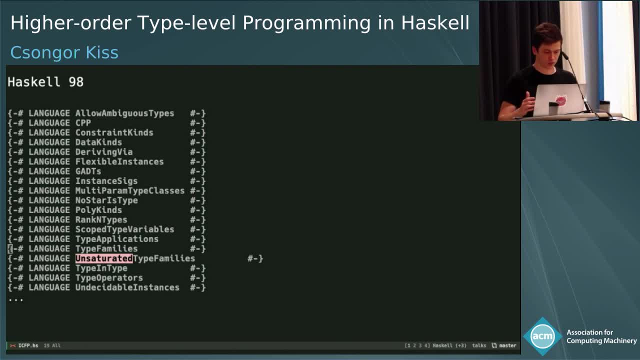 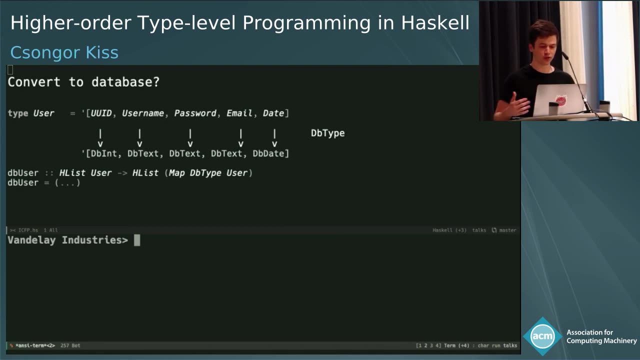 But luckily, unsaturated type families implies type families, so We're back to 98, so it's all good, It's all nice, Okay, so Right, so we reload in our new version of GHC, enable the extension, and it works out just great. 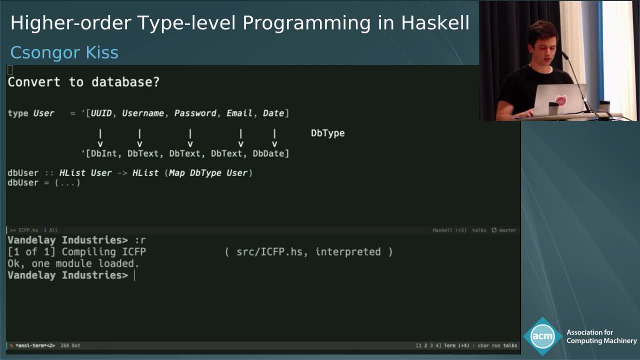 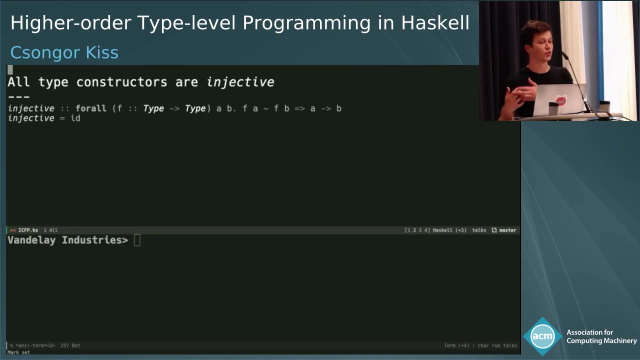 So we can. We can now do type-level higher-order programming And to check the type of this, the type of DB user I want to apply to Chris is indeed the mapping. So it all works out great, Is that? And okay? so as a sanity check, we need to make sure that we didn't break anything in the process. 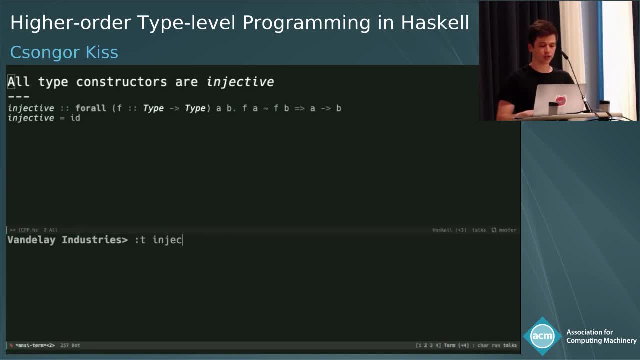 So what happens when we now try to instantiate injective with DB type? Well, previously it didn't work because of the saturation restriction And now it doesn't work because it's a normal type And it says: well, this thing doesn't fit in that hole. 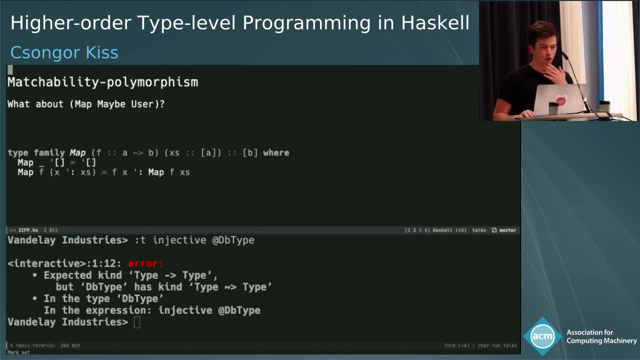 So we're still good. Now what about? So we can now use map to map functions or type families over lists. But we've kind of lost an ability in the process, which is that What if we try to map the maybe type constructor over this list? 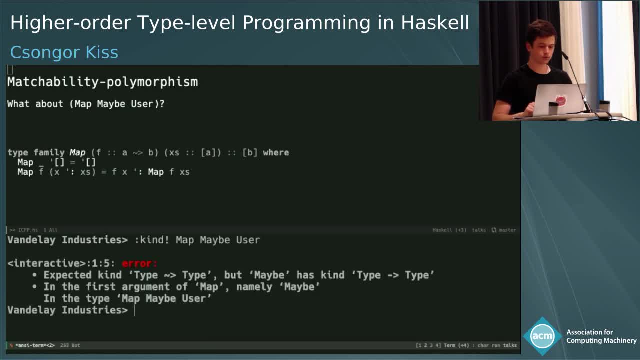 Well, let's try. Oh okay, so we get a kinder, which is to be expected, Because maybe It still has the matchable arrow kind. But clearly the kind of map expects a type family. So here's a second idea. 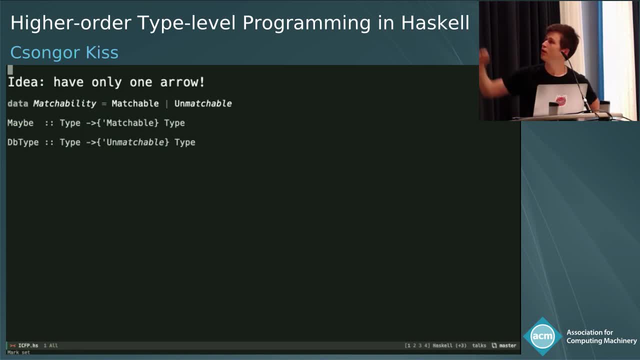 Instead of having these two distinct arrows, have only one arrow, which will then be indexed by its matchability. So we have this data type matchability, which can be either matchable or unmatchable, And so now the kind of maybe becomes type arrow, the single arrow with matchability instantiated to matchable. 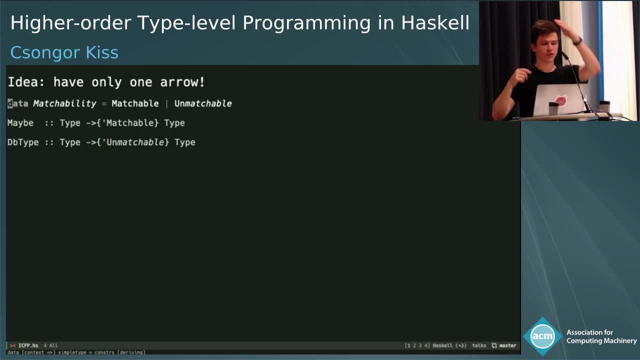 To type and DB type, type to unmatchable type, And I don't know what you're thinking. This looks really ugly. So we can introduce the matchable arrow and an unmatchable arrow as simply type synonyms with the relevant instantiations. 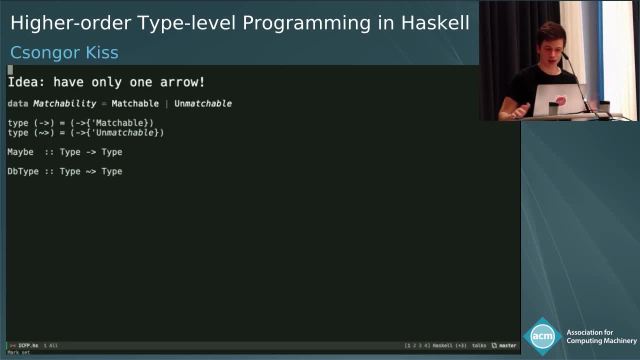 So we go back to how things were before, Except what this allows us now to do is to go to this arrow and replace it with a matchability variable. So now map is a function that takes either a type constructor or a type family, And let's try map DB. type user. 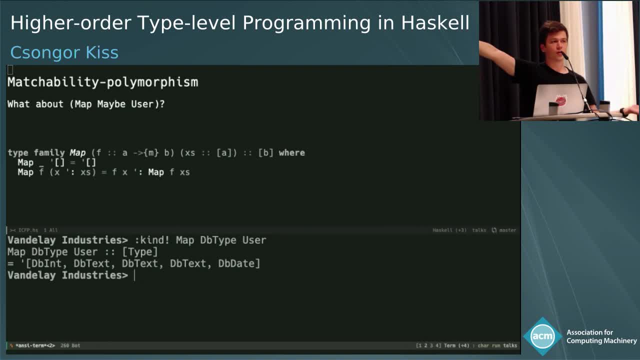 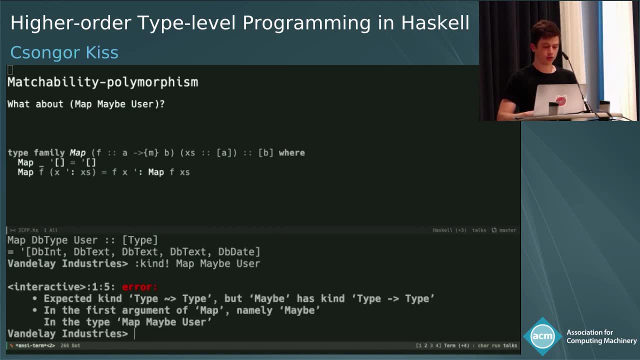 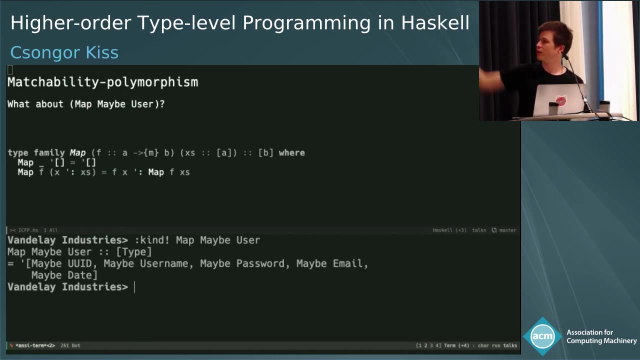 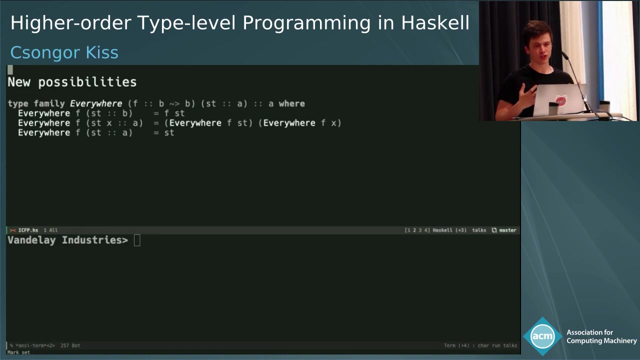 So in this case the matchability will be instantiated with unmatchable And if we do, maybe over user. I didn't reload the file, Always reload the file, Okay, Okay And maybe works Again, And because I don't have much time left, I'm not going to go into very much detail about how this function works. 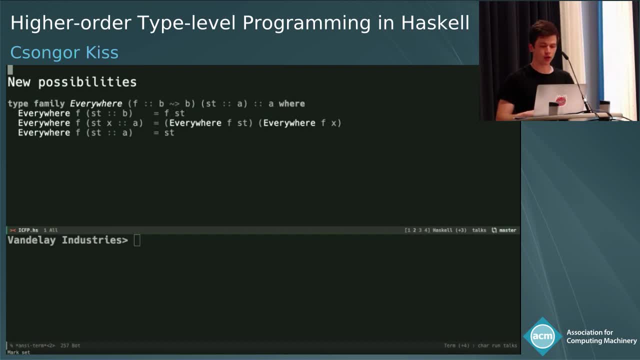 But just a glimpse of what else you might find in the paper. We can now, using unsaturated type families and some of GHC's more interesting type system features, we can do really, really, really nice and reusable generic programming at the type level for the first time. 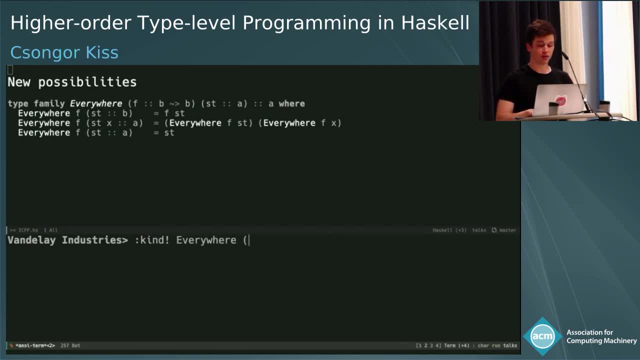 So I can say: I want to apply a function everywhere In a type where it can find an int, I want to add 10 to that type level int. So I'm going to just define a type level list of type level tuples of maybes, of nads. 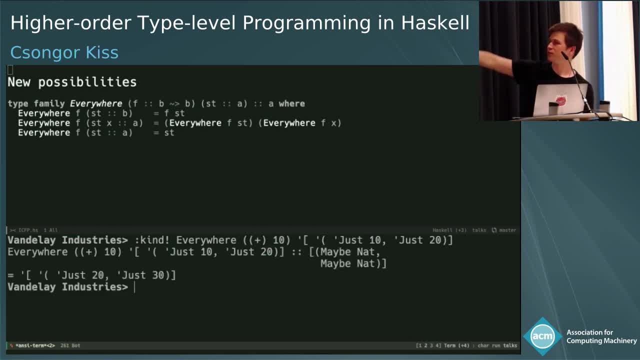 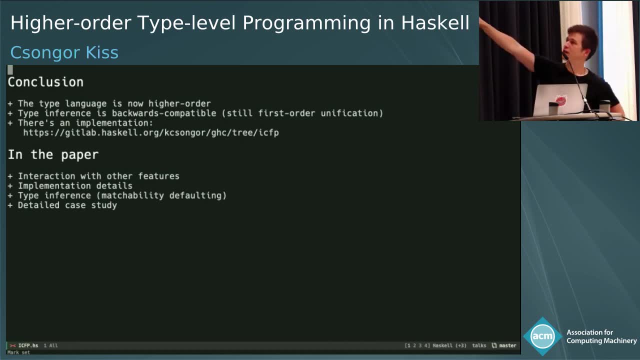 And see what happens. And it adds 10 to them. So if you want to understand this function, go look at the paper. So just to conclude, we just made the type language higher order in a way that type inference remains backwards compatible. 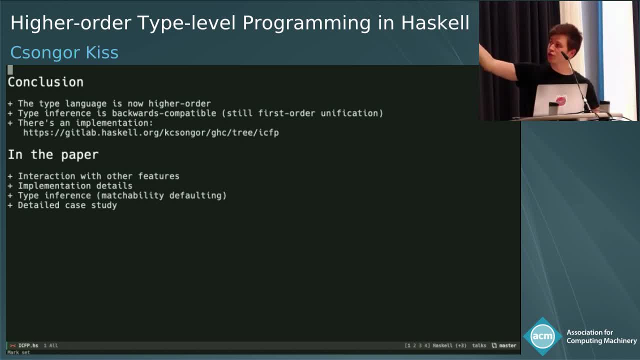 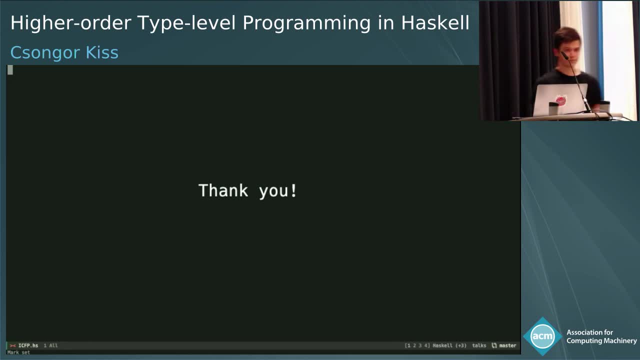 We're still doing first order unification. We have an implementation of this work which can be found at that link, And you can find more details in the paper. Thank you very much. All right, Thank you. I think I was mostly impressed by how you. how long did you practice to get the keystrokes and sync to the video? 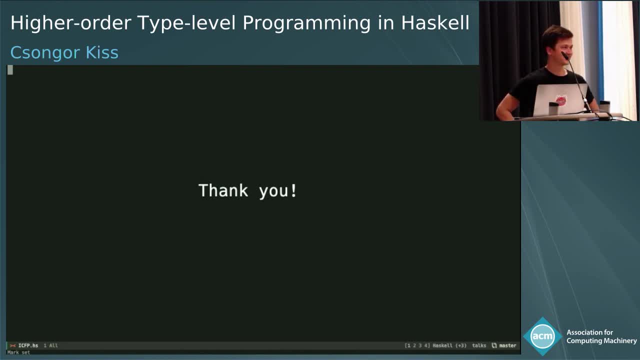 Okay, never mind. So there's one question online that maybe was answered by the last slides: Is there a sub-kinding relation between the two kinds of arrows? Yes, So the answer is: the two kinds of arrows are just now instantiations of the single arrow, which is indexed by its matchability. 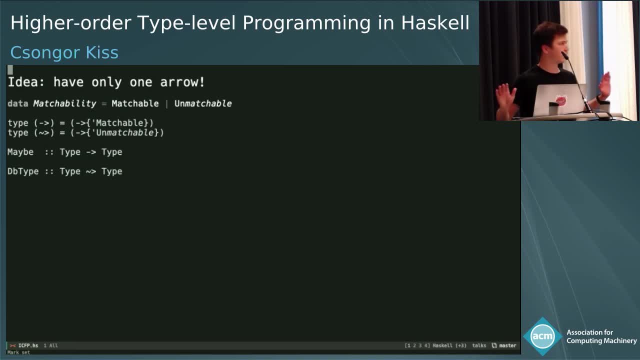 So that's the connection. Okay, but they're not sub-kinds of each other, but rather they're both sub-kinds of the polymorphic one. Oh, there's no sub-kinding relationship. Yeah, Okay, Do we have any real-world person question? 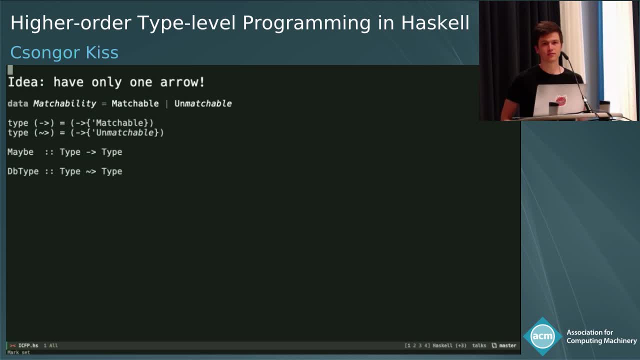 Yeah, over there. So what's the story with type errors? Do we have to teach beginners about matchable and unmatchable arrows before they can understand things? Oh, type errors, Right. So if you're not using this fancy type system feature, then all you're ever going to see is the old normal type error. 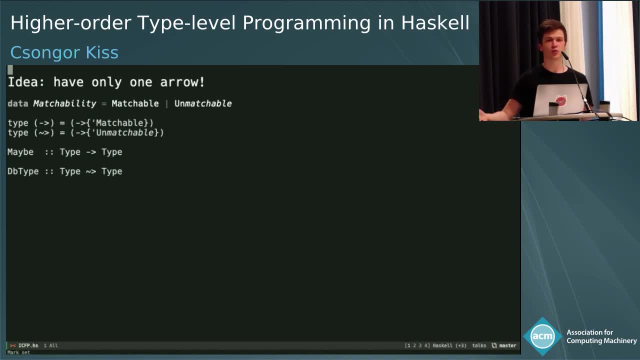 So type error, the type arrow. So in type errors you shouldn't see a difference. Okay, And if you're already using these advanced features, then good luck. All right, This must have been one of the clearest talks, because there's a surprisingly small number of questions. 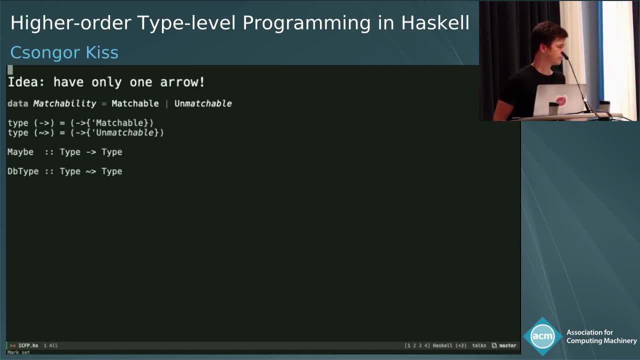 Oh yeah, There's one over there. This kind of looks like an effect system at the type level, right with polymorphic instantiation. Do you actually ever need the generality of that, or would sub-kinding or sub-typing at the effect level just have been enough?